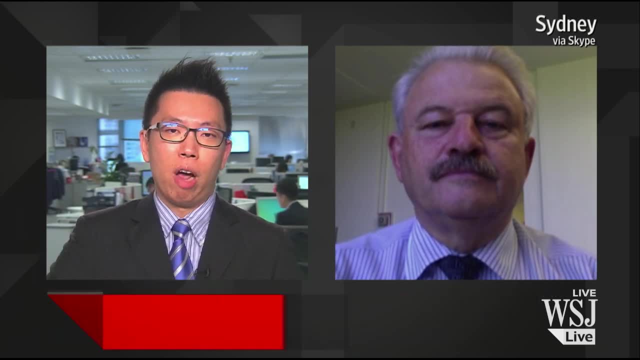 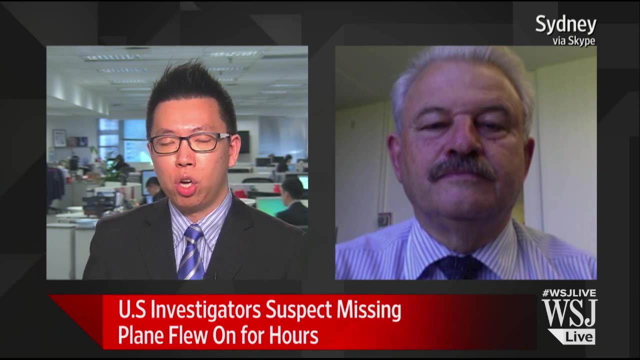 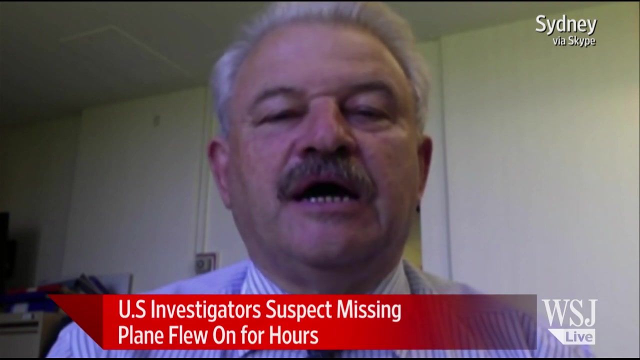 other theories that there was a catastrophic break of the aircraft in the air. What's your assessment of the transponder issue? just no longer transmitting What could have caused it? Well, in line with the fact that there's no communications as well with the pilots. 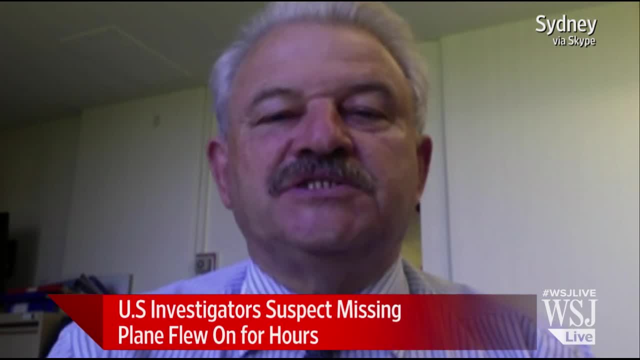 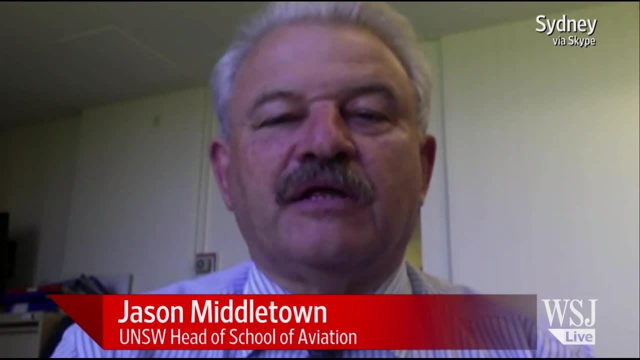 that suggests, if the airplane is still flying, that there was a fairly significant malfunction of the entire communication system and probably disablement of the pilots as well. So you can think of ways that might happen. Each of them is unlikely, but then of course, 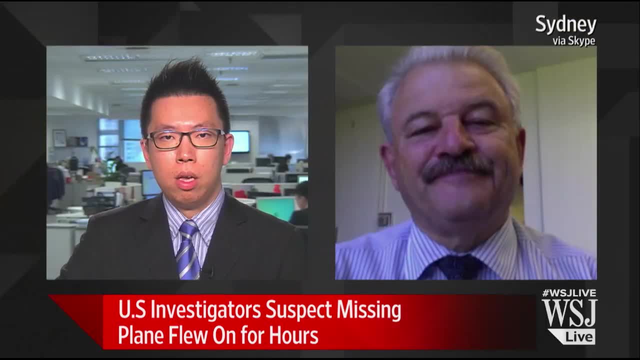 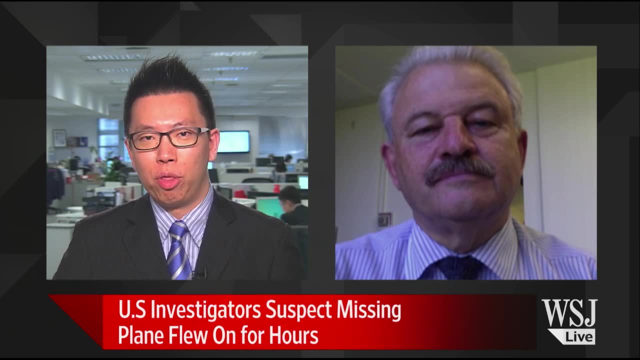 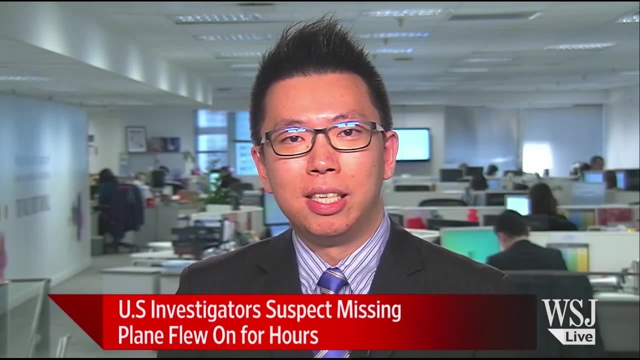 every scenario we're thinking of at the moment is unlikely. That definitely. I guess with this latest story the search parameters may be much farther than what the Malaysian and other authorities are looking for this jet. But in your opinion, in your assessment of the very limited data, 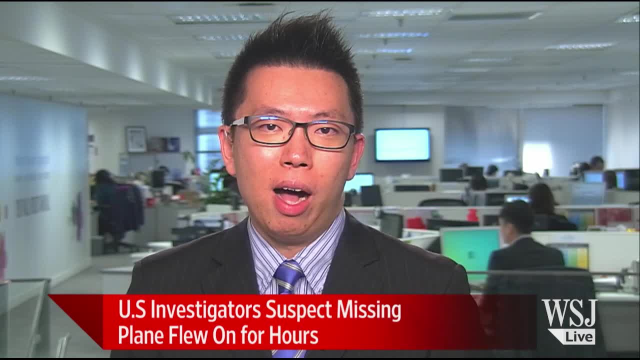 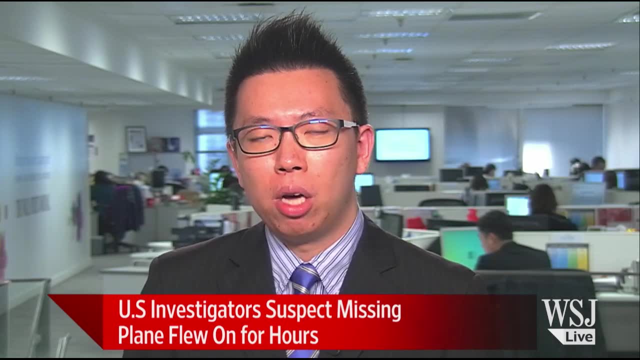 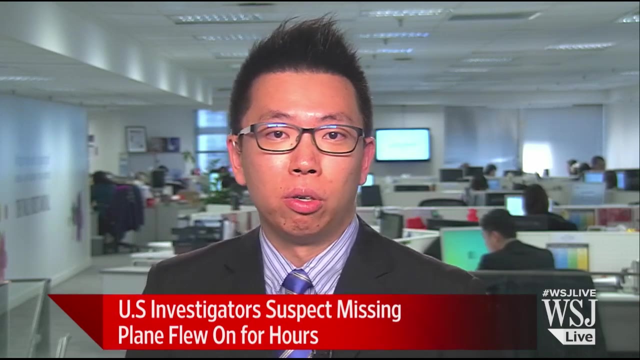 that we are provided at this time, what other scenarios, or what are the more compelling scenarios that you see, as an expert in aviation, to be possible causes or what has brought this plane or made it disappear for so long? Well, you've really got two choices. 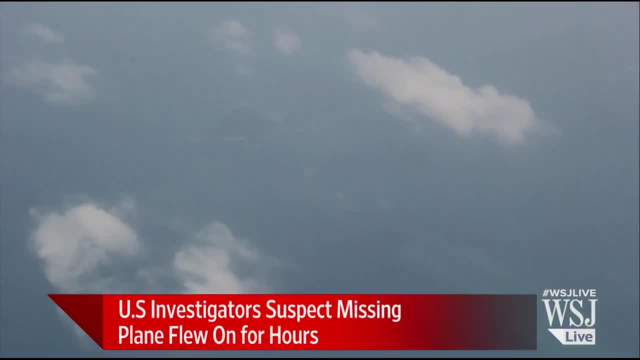 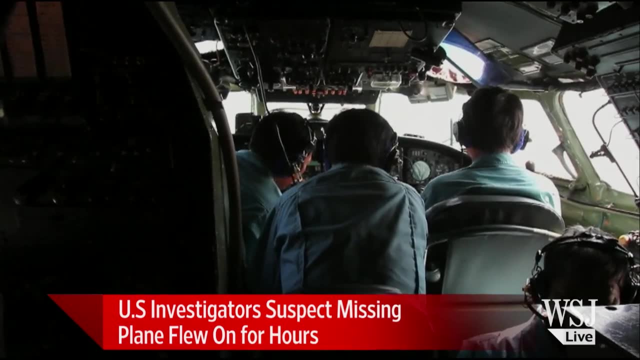 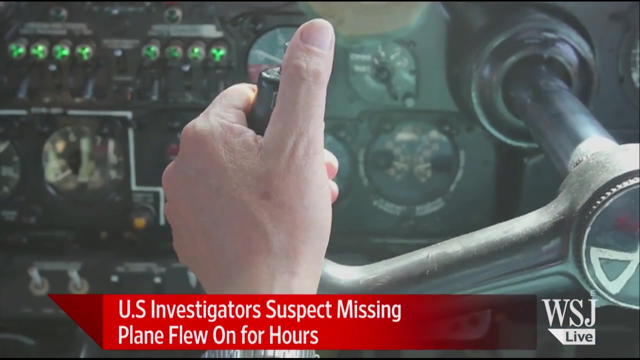 It's some sort of catastrophic malfunction in which there's no sort of illegal activity that played a part, just systems failing and failing terribly badly in a peculiar set of circumstances, Or there's some sort of illegal intervention that could be someone on board or could be. 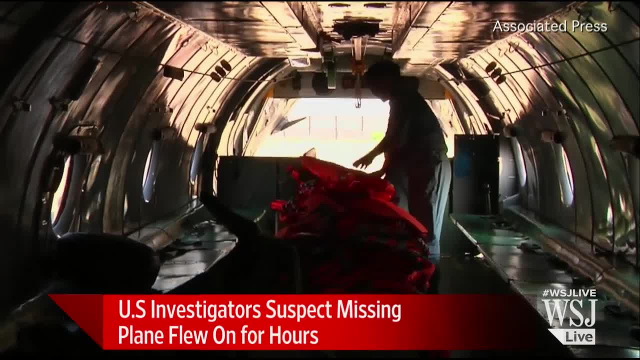 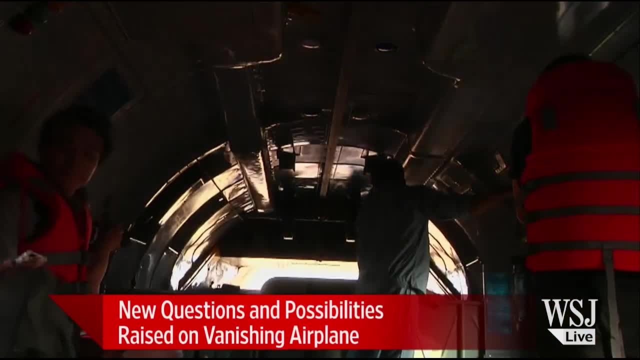 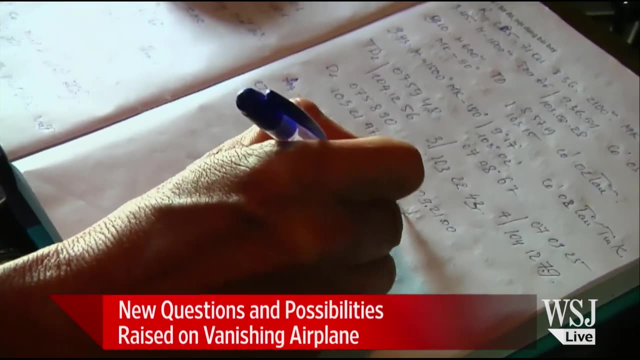 for example, explosives that packed in the cargo which again caused such a serious set of malfunctions that the airplane and the pilots are incapacitated. So whether it was human caused or otherwise, certainly it must have been some very serious malfunctions. 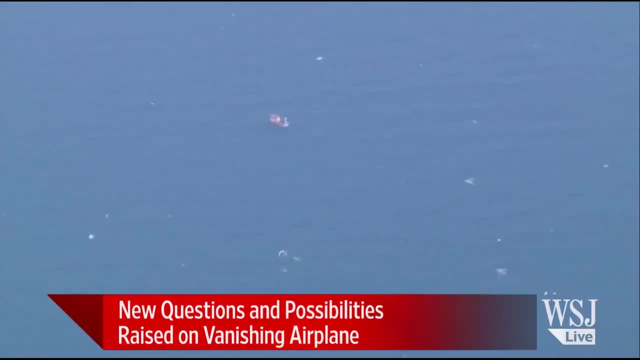 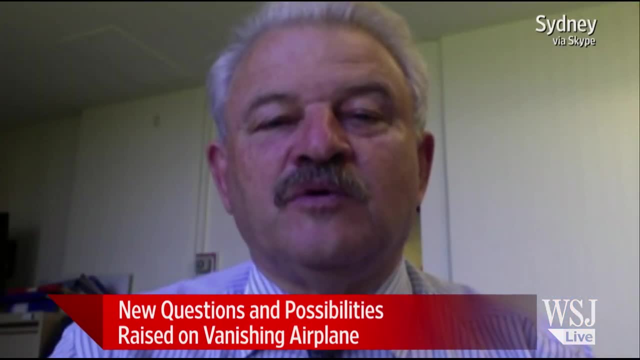 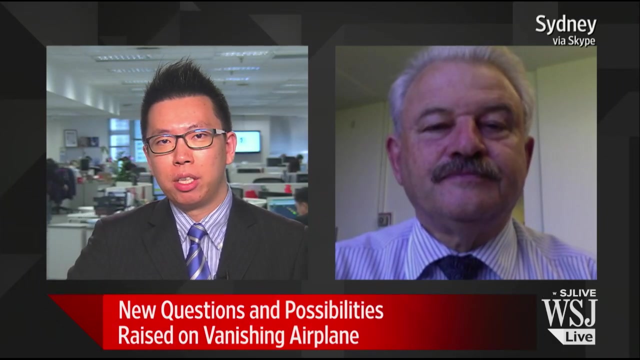 To have the airplane flying is really, really curious as well, because anything that would seriously cause those malfunctions probably would affect the autopilot as well And the airplane would crash into the ocean. Professor, I'd like to go back to the question on ACARS.